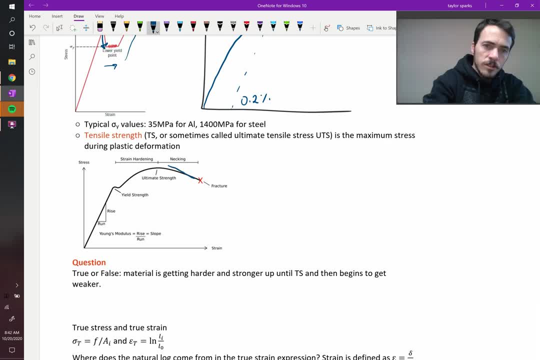 Notice that the stress actually starts going down. It's still, it's like it's deforming still, but the stress to make it deform is going down, down, down. So this is your maximum, or your ultimate tensile strength. That's the maximum that it can ever withhold. 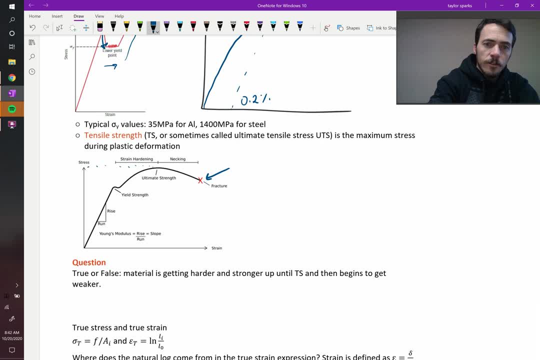 And after that it goes down, And then you of course have your stress at fracture. So you could have a stress at fracture as well. Okay, Now quick question. This plot looks a little bit funny, doesn't it? 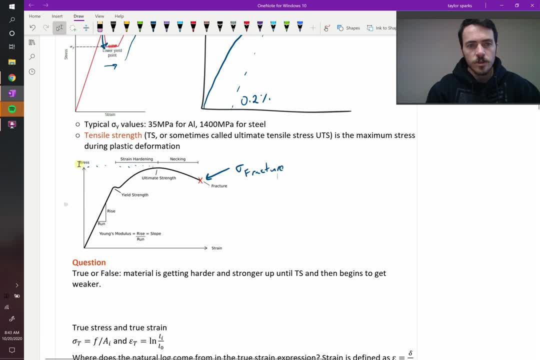 Right, It makes sense that if you apply More and more stress, you get more and more strain, And so this general upward curve makes sense. But why would it ever start turning down right? So, true or false, The material is getting harder and stronger, up until the tensile strength TS. 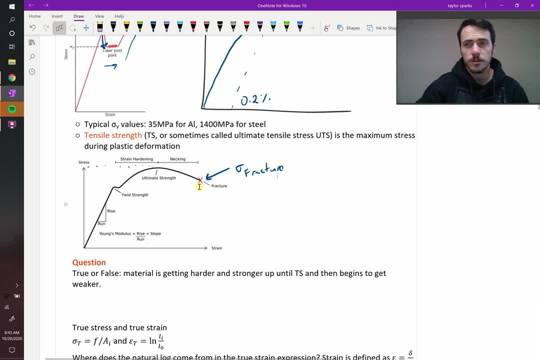 And then it becomes weaker, right Since it's going downhill, True or false? So it's a bit of a trick question. As you deform materials, they always get harder and stronger, So why would it look like it's going down? 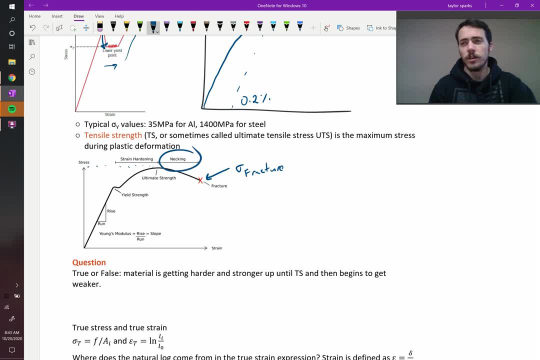 You get right here, it's labeled- You get Necking occurring. Necking in your material is when you get localized plastic deformation. So instead of the whole thing deforming sort of uniformly, you get local deformation. So let's say this is your dog bone. 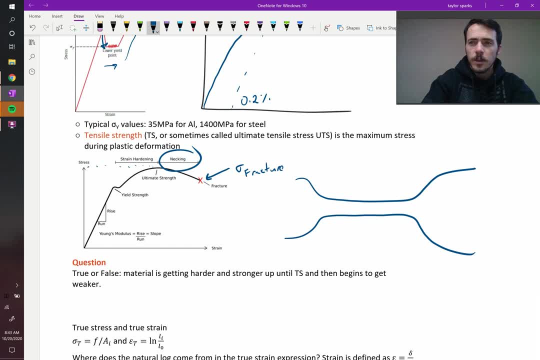 Right, That's before you bend it. But you can get localized deformation where maybe it looks like this: Right, This region right there basically gets further drawn down. That's called necking. OK, We'll show you some pictures of that in a minute. 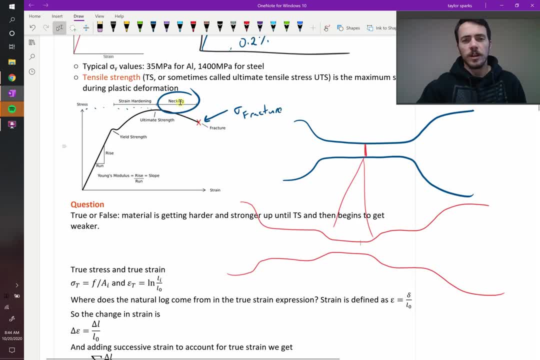 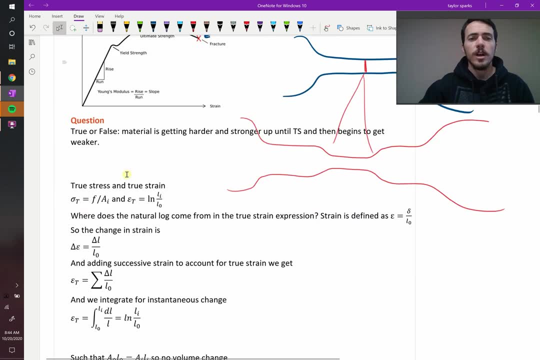 Because of that, what you really need to do in a plot like this- to plot it accurately, to get true stress- is you need to calculate true stress and true strain. Here's how you do it. True stress is defined by the force divided by your instantaneous area. 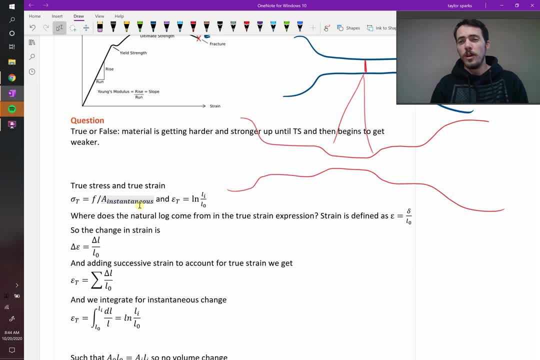 You're instantaneous area. What do you get under Anuv? You're instantaneous or at any given moment. you take that area, not the area that you started with, because those are different. Because if it draws down like this cross-sectional area, right there. 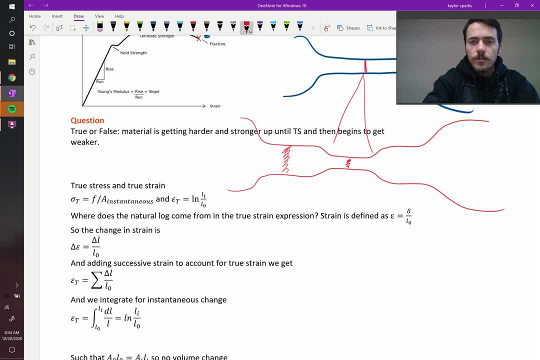 is way smaller than what you started out with, right, And then your true strain would be the natural log of your instantaneous length divided by your initial length. all right, And where does that come from? We've done the derivation here, but I'm going to skip it for this class. 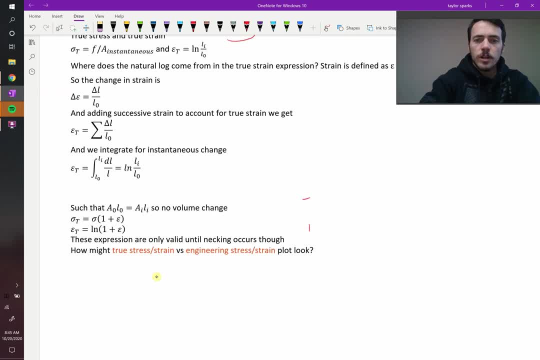 You can take a look at it if you want. So an easy way to calculate this. your true stress sigma t is equal to the stress that you think you applied, because that's divided by your initial area, multiplied by 1 plus epsilon. okay, 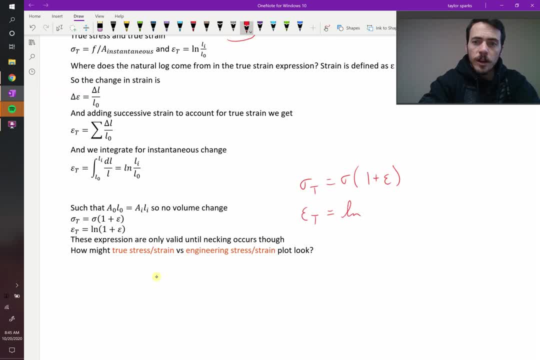 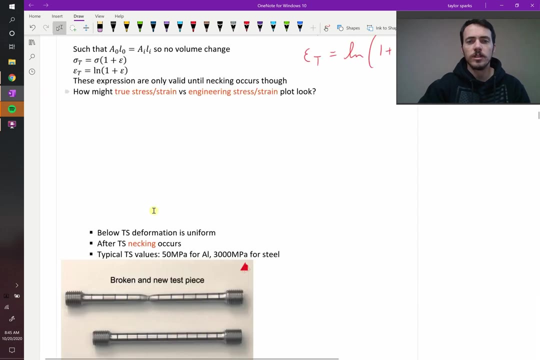 And your true strain is going to be equal to the natural log of 1 plus your strain. okay, Now, these expressions are only valid up until necking occurs right. Once necking occurs, all bets are off. So how would a true stress and strain plot look different? 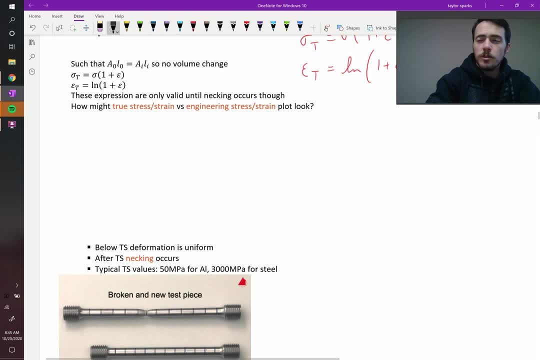 than an engineering stress and strain plot. Again, engineering is when you divide it by your initial area and true is when you divide it by the instantaneous area. So, again, if we plot stress versus strain, we know what engineering stress and strain looks like. 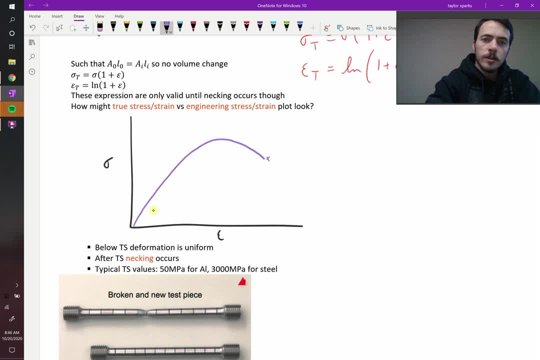 It goes up, it comes down and then it breaks right. So true stress and strain would keep on going up until it broke. all right. Yeah, It would keep on going up because you're taking into account instantaneous area, right to get your true stress. 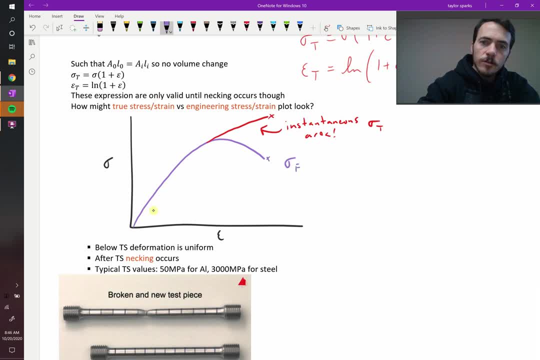 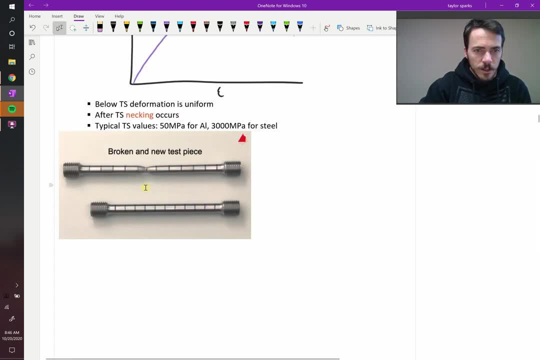 as opposed to your engineering stress sometimes sigma e. okay, So what are some examples of this necking? Here you can see it. These markers were equally marked. I think they were every 1 centimeter on this bar And then, when they pulled it, you can see that between this marker. 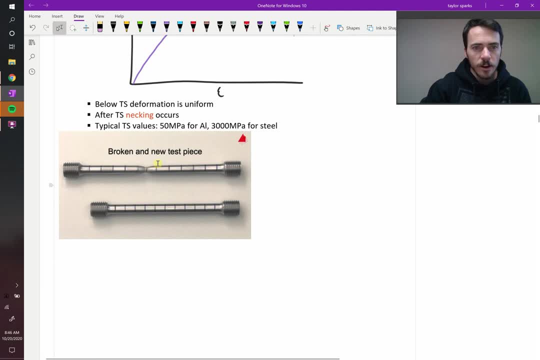 and that marker it's now like double the length because right there you've got additional, you know, deformation that was localized deformation occurring in your material And then the break obviously occurred there because look at your cross-sectional area, It's much smaller there than over here, so it has a higher stress state there.